managed to tick off a lot of tasks. 1. Declutter your workspace. The first step to time management success is having an organized workspace. The second step will help you stay on track rather than swaying to and from tasks, and it will also give you a great sense of achievement when you've managed to tick off a lot of tasks. The first step to time management success is having an organized workspace. The second step will help you stay on track rather than swaying to and from tasks, and it will also give you a great sense of achievement when you've managed to tick off a lot of tasks. 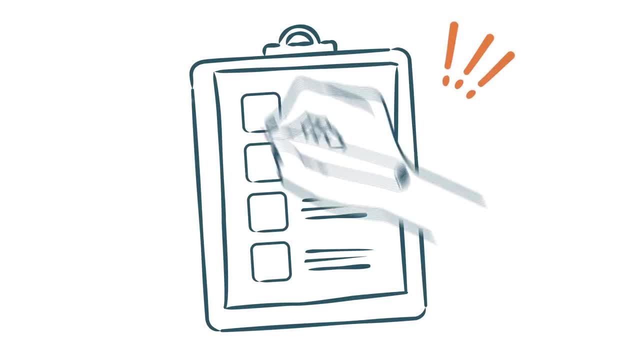 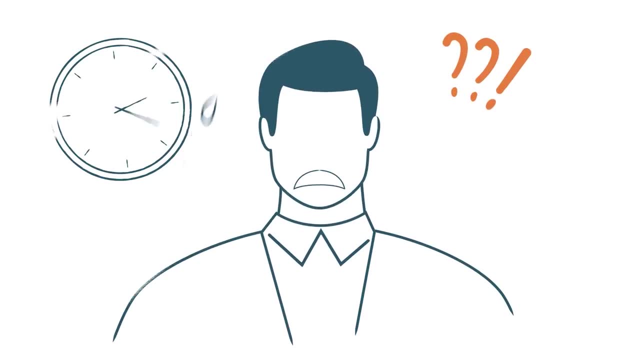 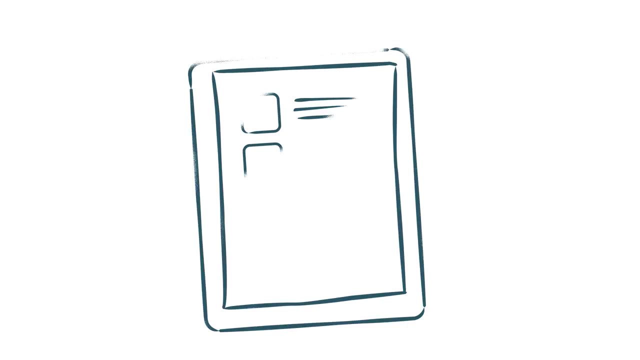 The best way to create your list is to analyze your tasks towards the end of your shift and prepare for the following day. That way, you won't waste time in the morning, when you're most productive, on something minor like a list. 3. Prioritize- Now you have your list of duties. you'll need to rank them in order of priority. 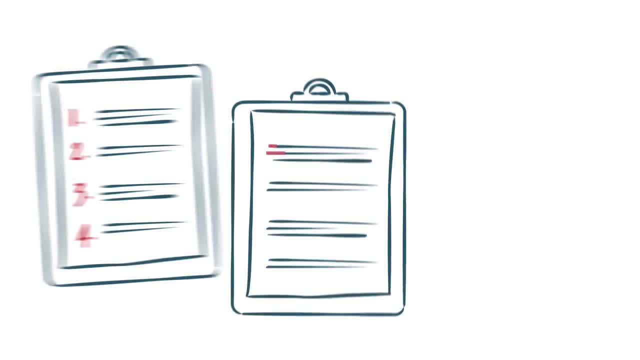 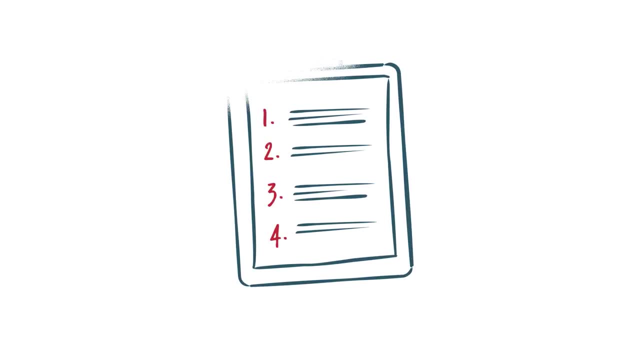 The way you do this is up to you. You could use a numerical ranking system, highlights or mental notes. What's important here is to understand which is the most urgent job and get that out of the way first. 4. Set achievable goals. A great way to stay motivated is to set achievable goals. If you have 20 difficult tasks. 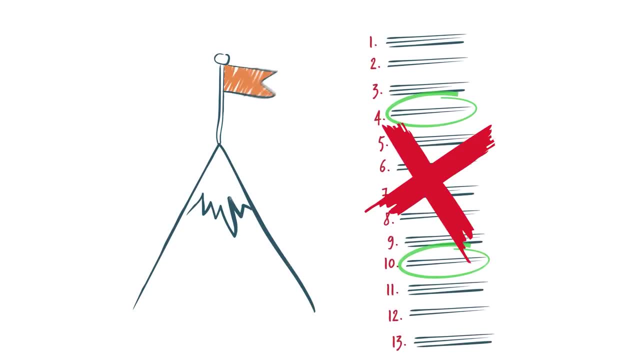 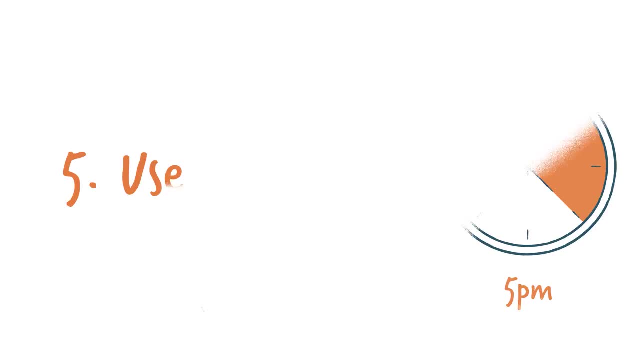 it's apparent that you won't achieve them all in one day. Therefore, be realistic when prioritizing and creating your list so that you don't get disappointed when 5 pm rolls around. 5. Use organization apps If you're tech-friendly. an. 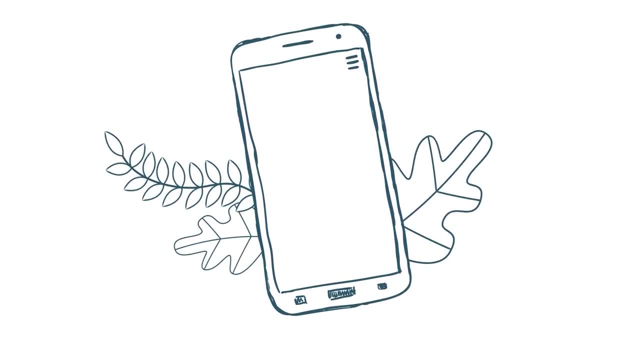 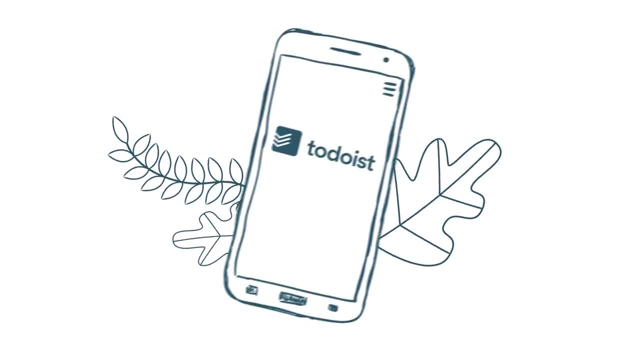 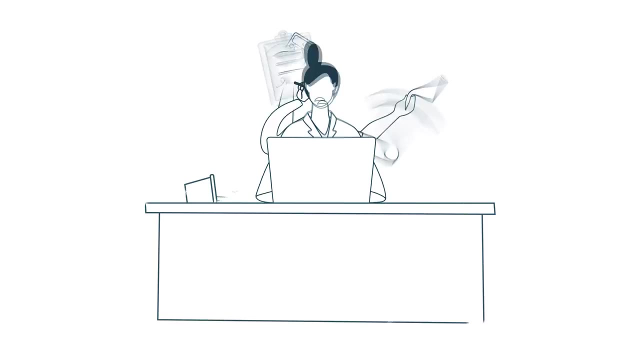 organization app is what you need in your life. You could use a project management tool like Trello to keep your tasks visible and your workflow clear. On the other hand, if you want a simple checklist, Todoist is your perfect match. 6. Don't multitask. Many people assume that multitasking is a great skill to have, but if you're not able to work fluidly, 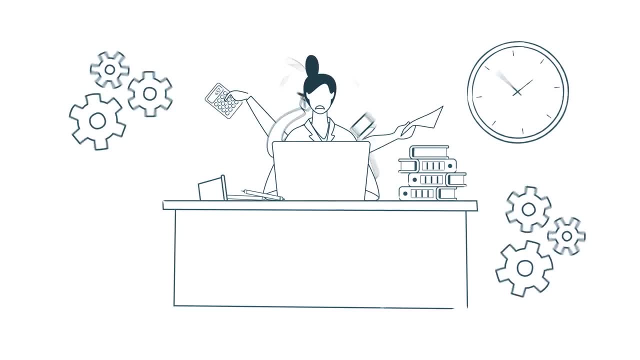 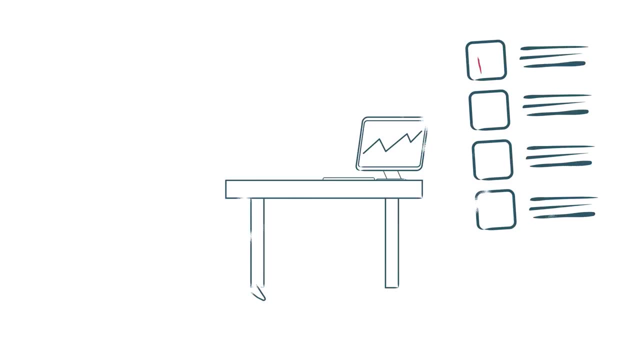 you'll end up bouncing from tasks and wasting time in between. This can also lead to careless mistakes and forgetfulness. 7. Reward yourself When you finish the big task. why not reward yourself with a treat? This could vary depending on your interests. 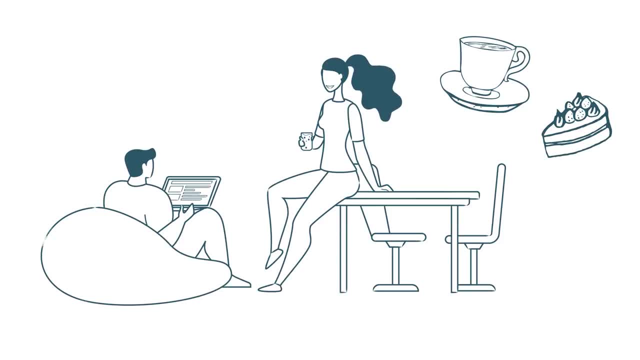 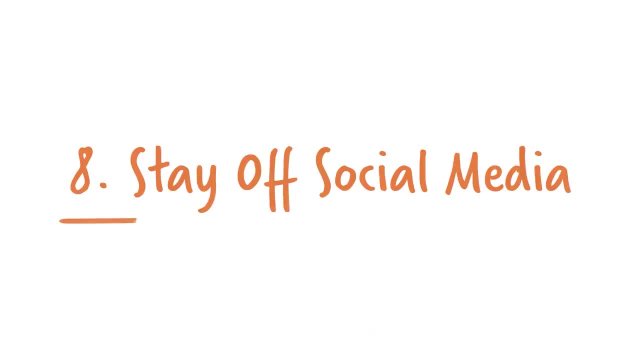 You might want to order a coffee, a cake or have a ketchup with your favorite co-worker. Just don't overdo it and have 10 cups of coffee a day. That won't help anyone. 8. Stay off social media. 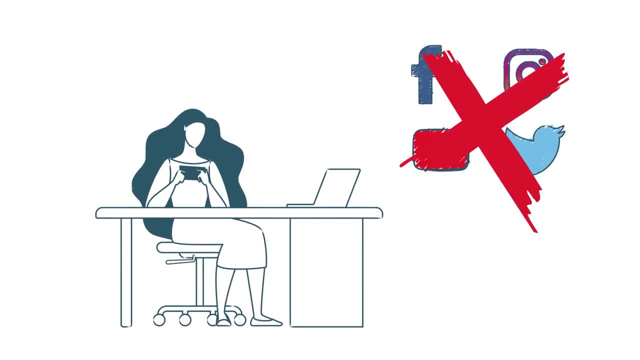 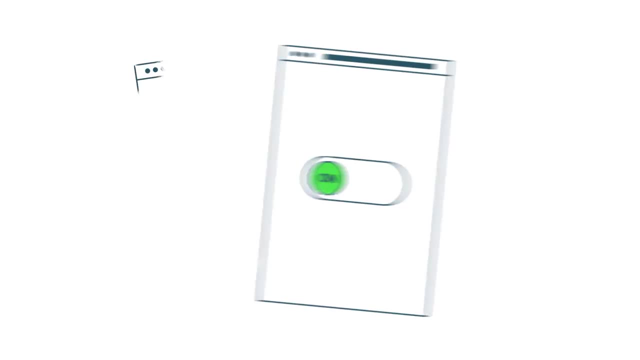 Unless you work in marketing. limit your time on social platforms when you're trying to get jobs done. If you really can't resist looking at every notification, put your phone on flight mode or download a social media blocking app. 9. Audit your time.